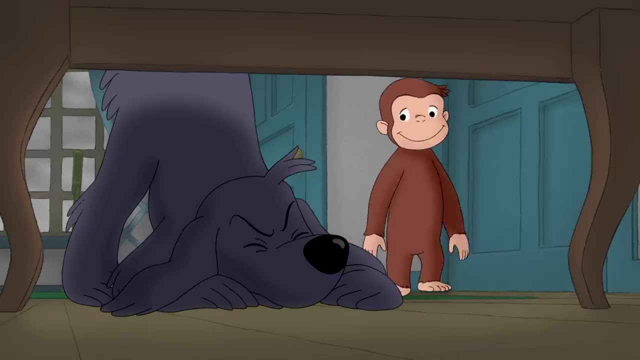 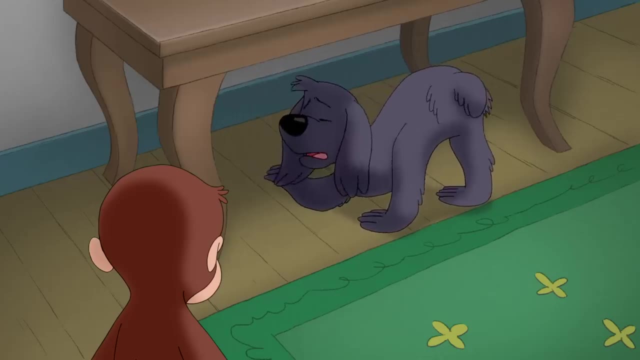 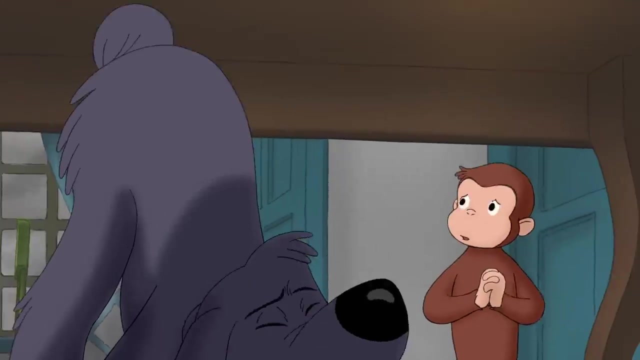 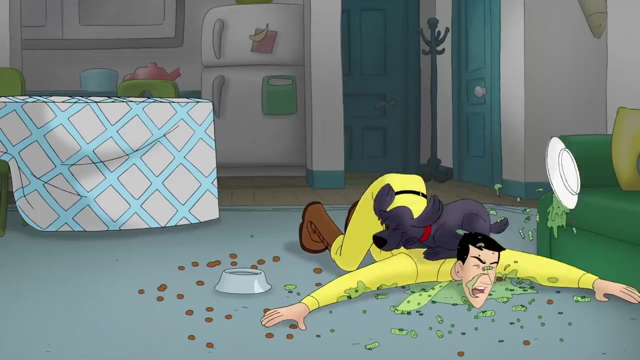 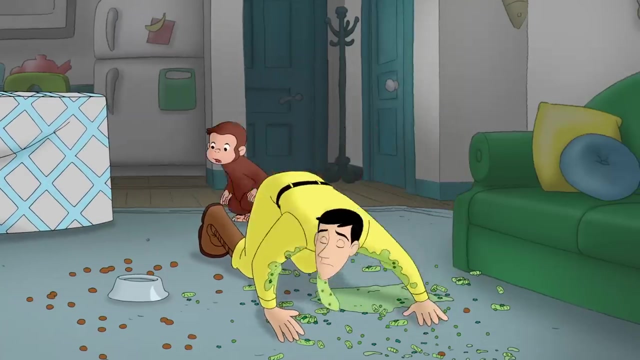 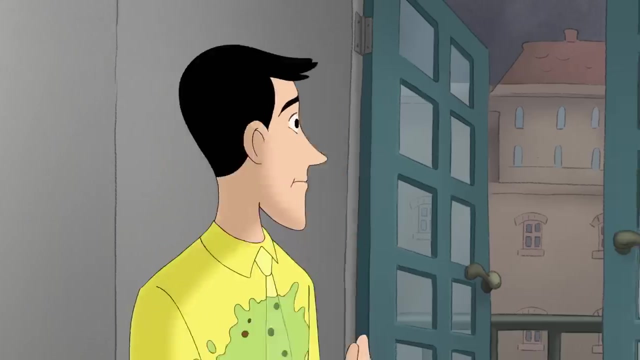 This was also not a very good place to hide. Why was Charky so afraid all of a sudden? It's a miracle I didn't get any on my shirt. Oh, Spoke to Zoom. She must be afraid of storms. Lots of dogs are. 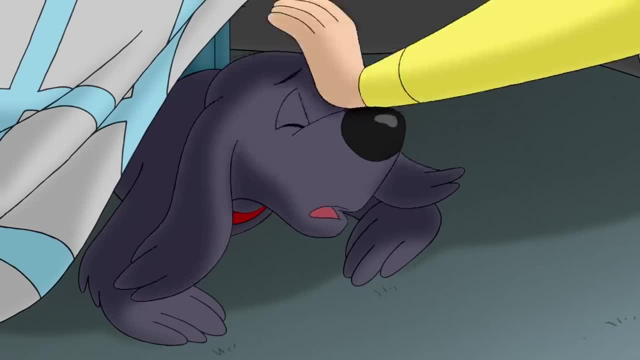 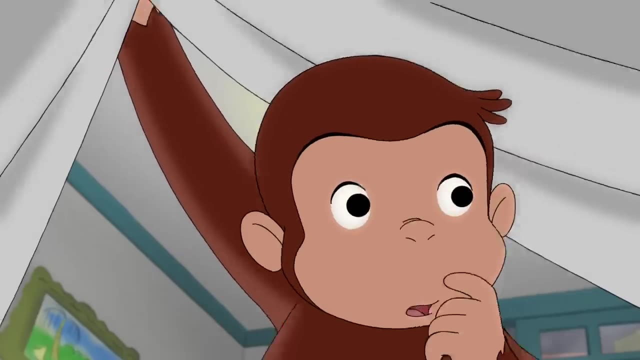 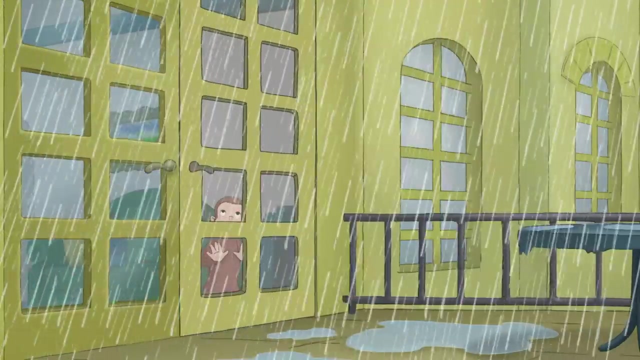 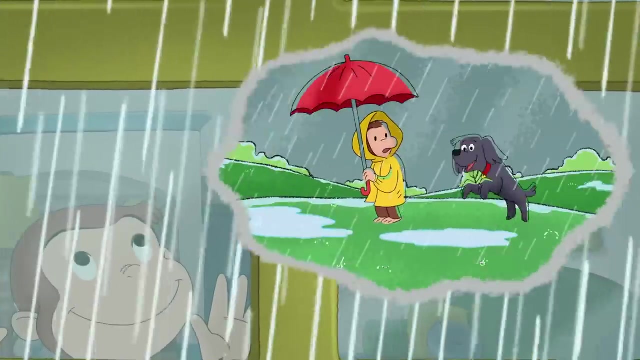 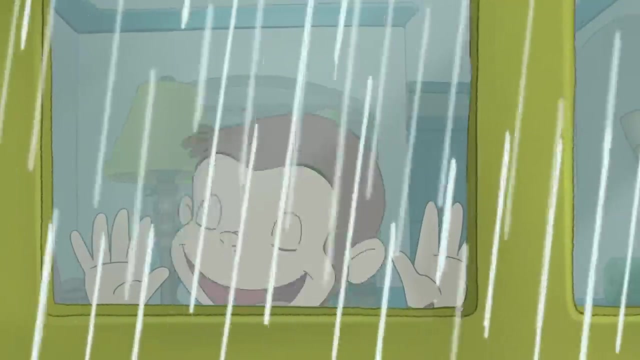 Oh, poor Charky, We're here with you. George wondered why Charky was scared of storms. He thought they were kind of exciting. Maybe Charky just didn't like all that rain. No, Charky loved any excuse to get wet. 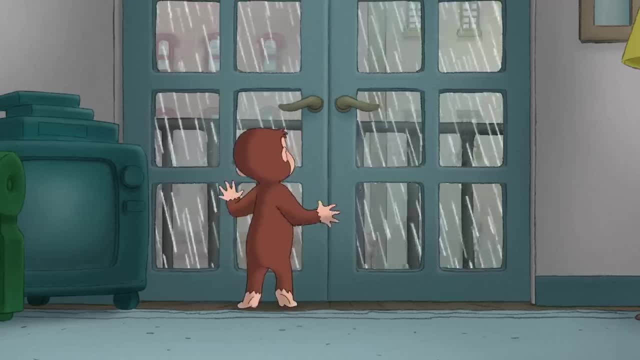 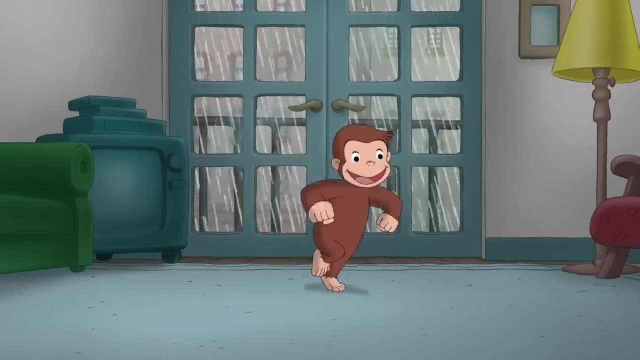 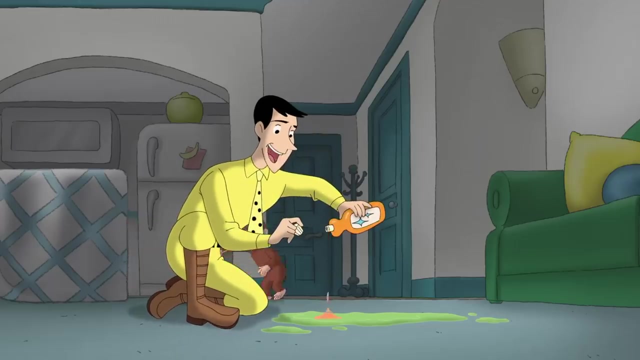 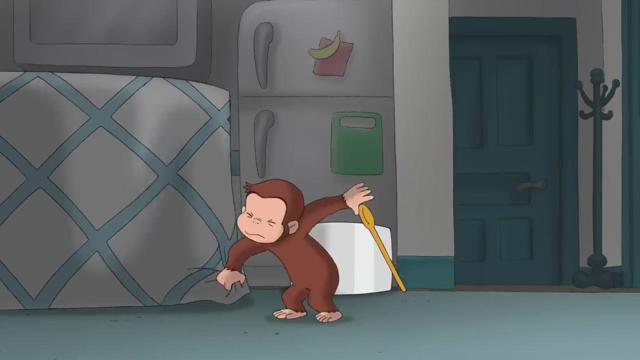 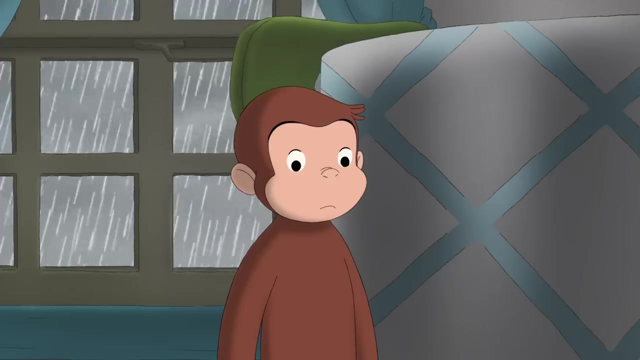 It had to be something else. Could it be the loud noise the thunder made? There was only one way to find out: A little dish soap should get this out. Nope, It wasn't the loud noise either. What else happened during a storm? 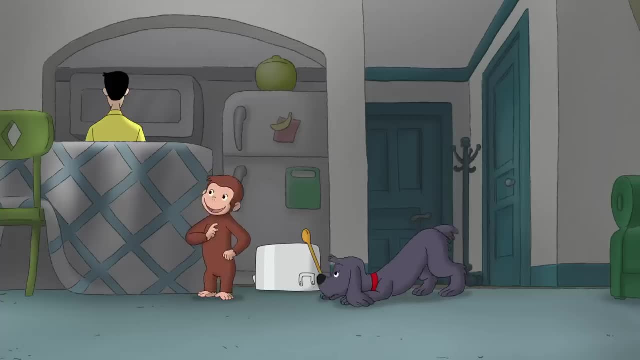 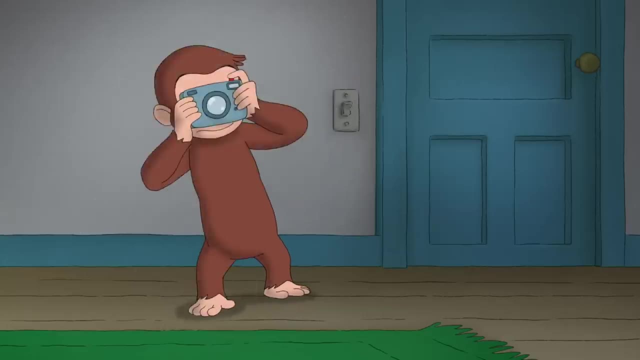 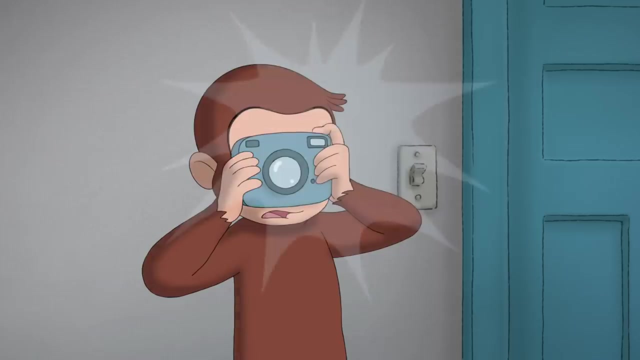 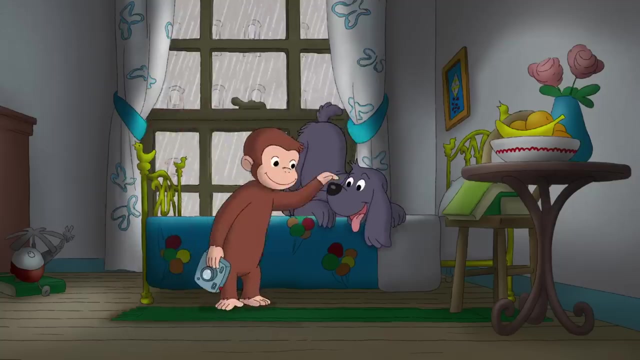 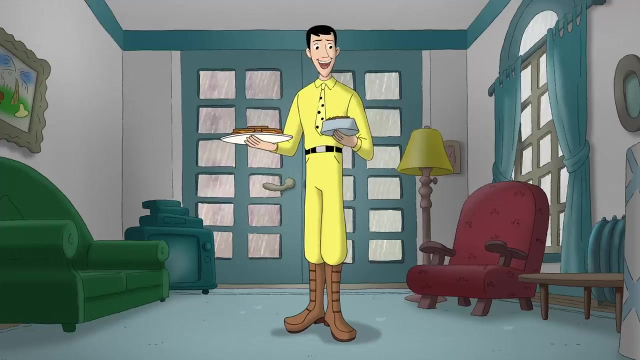 Ah-ha, Lightning, Lightning. Nope. Charky wasn't afraid of flashes of light, It was more afraid of the rain. It was more afraid of lightning and swarms of storms. No, it wasn't Except that kind. 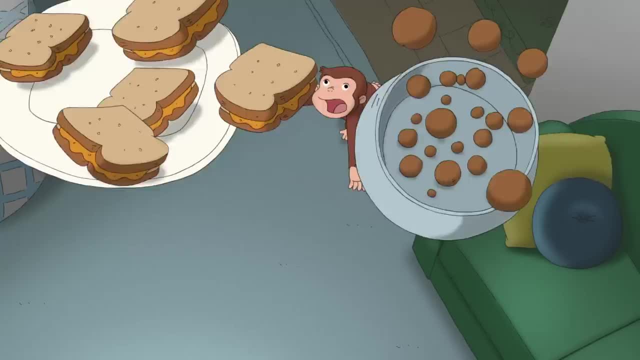 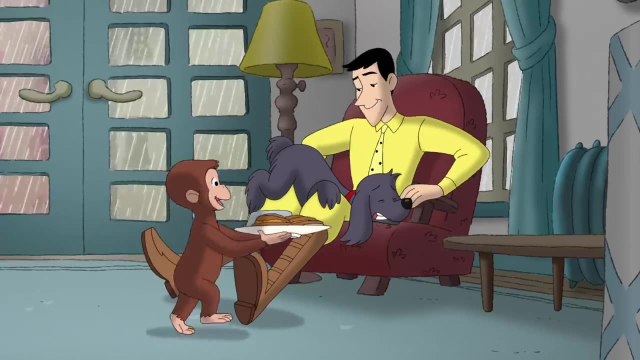 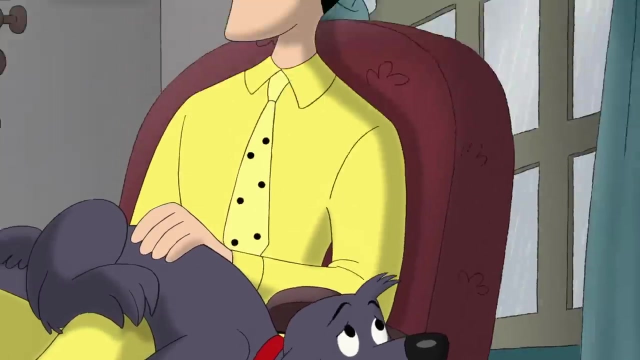 OK, more kibble for Charky and peanut butter and banana sandwiches for us. Ow Oh, Oh. Hey, I'm so over Meow. Ah, Oh, Oh, Oh, It seems like the storm is getting closer. 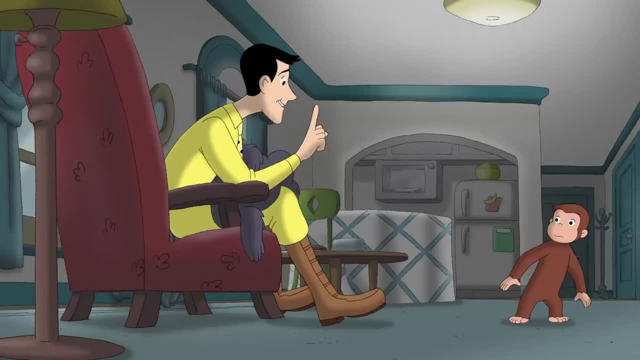 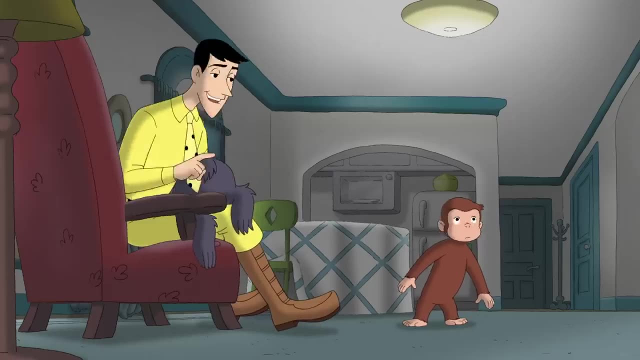 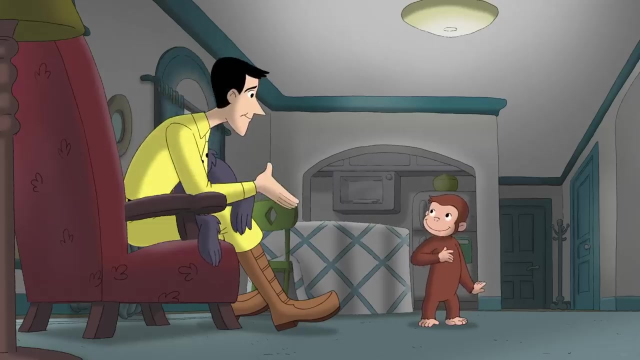 Yeah, you can tell how close or far a storm is by counting the seconds between the lightning and thunder. Quick start counting One, two, three, four, five. The last time I counted it was six seconds, so it's getting closer. 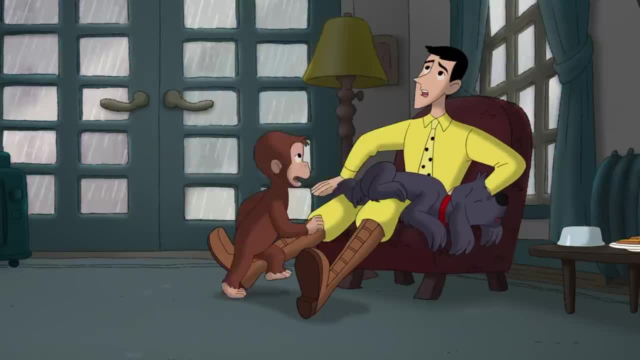 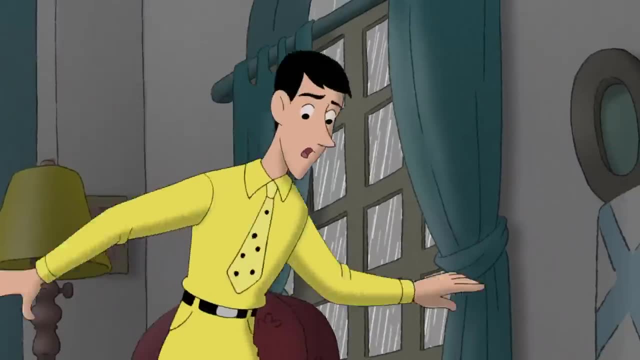 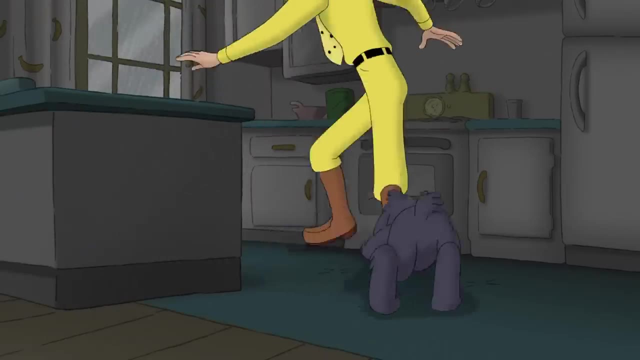 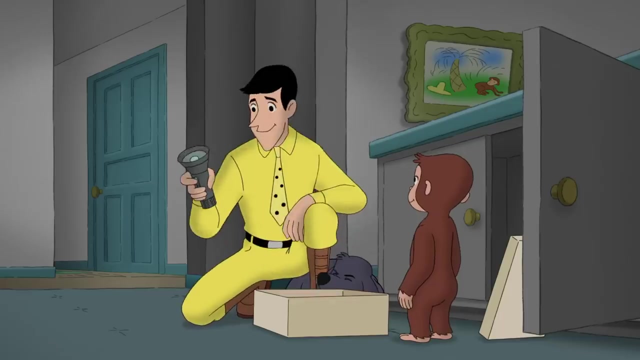 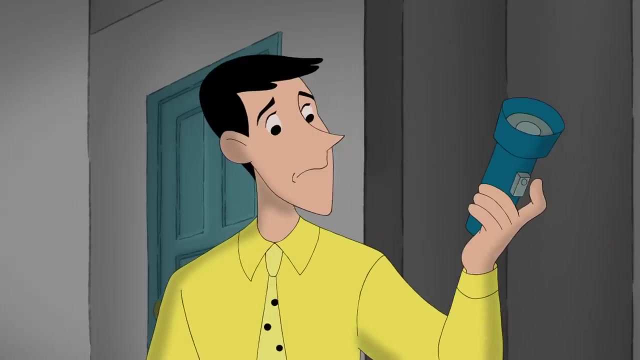 But don't worry, we're safe in here. It's okay. it's okay, The storm just knocked out the power. I'll get some flashlights. Well, we'll get there eventually. Uh-huh Huh, George, did you? 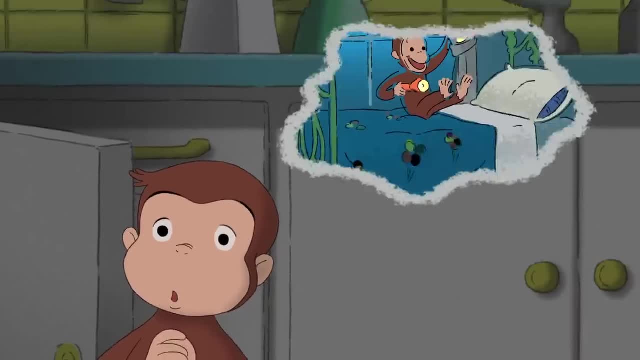 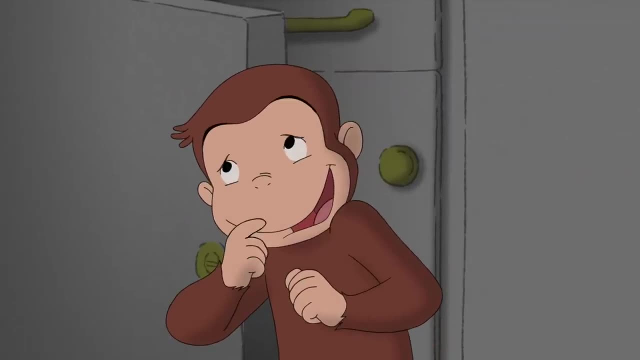 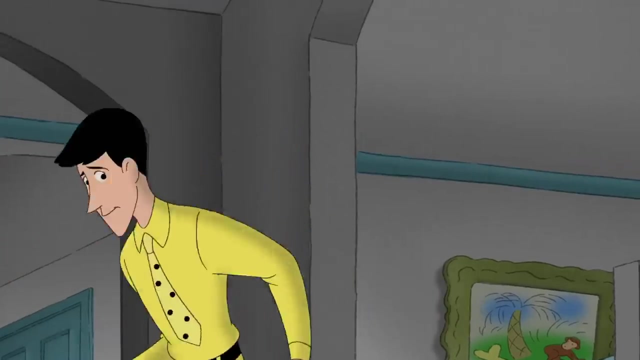 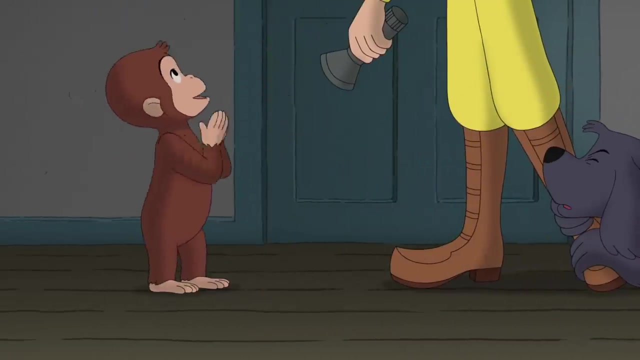 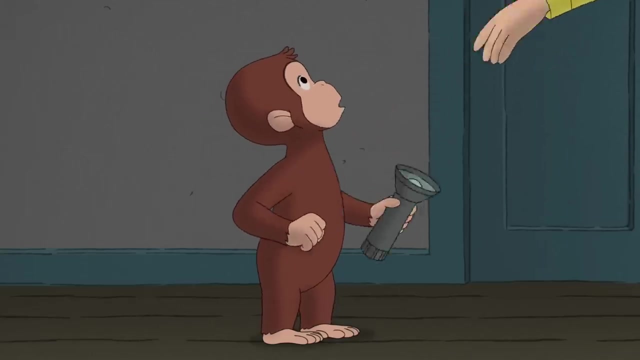 Did you use up the batteries playing with the flashlights again? I'll go ask the doorman for some batteries. Good idea. Oh, it's his lunch hour so he might be in his apartment. Oh, Ah-ah, Hmm. 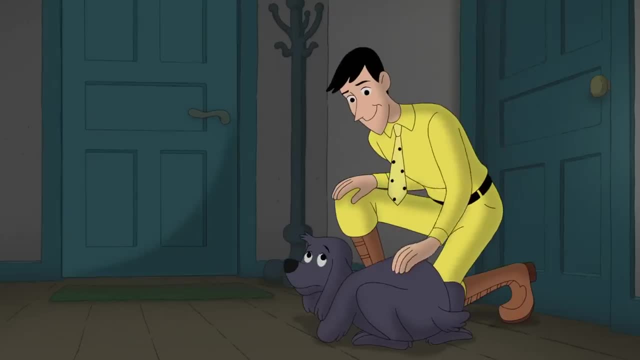 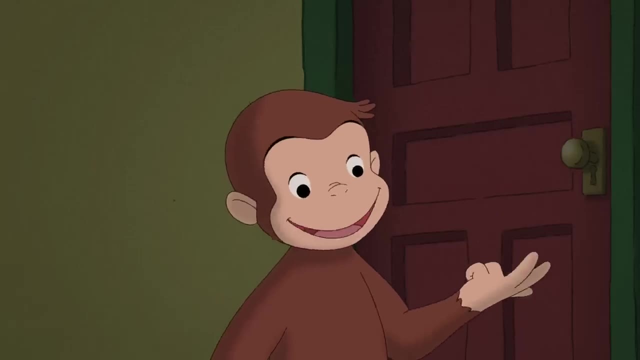 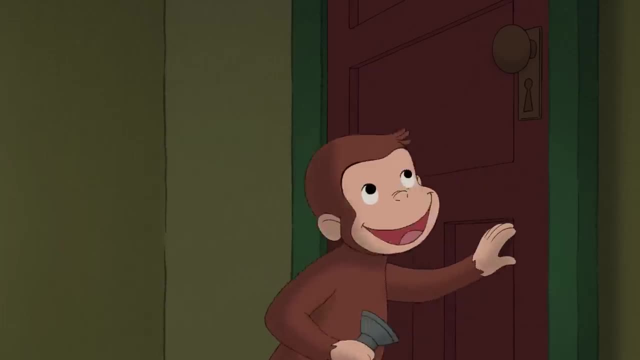 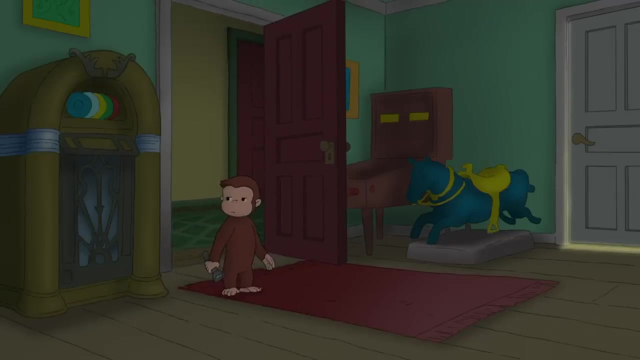 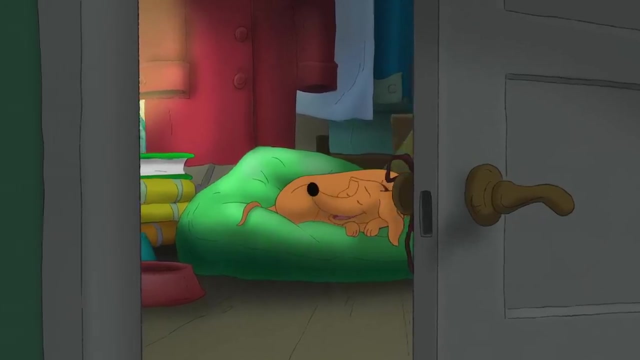 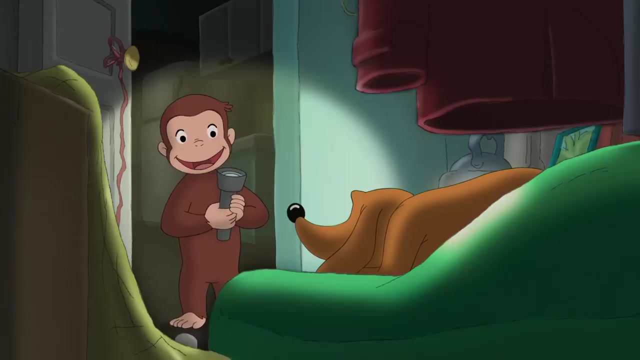 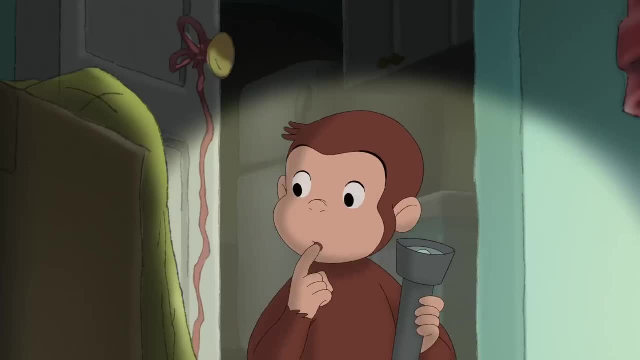 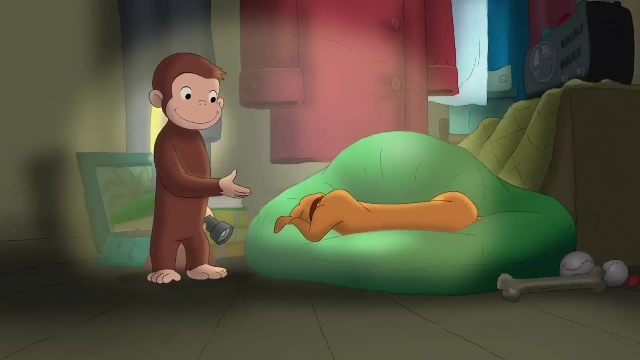 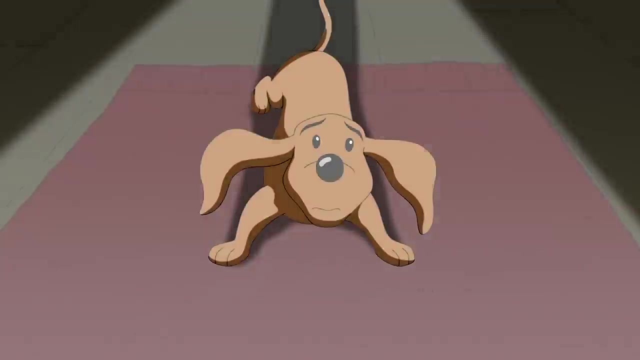 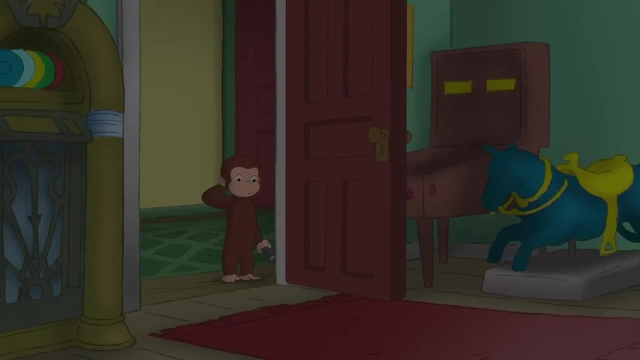 In fact he didn't even notice it. Maybe Hundley could tell George how to keep Charky calm during the storm. Hmm, Huh, So Hundley was afraid of the storm. Oh hi, George, Is the doorman home. 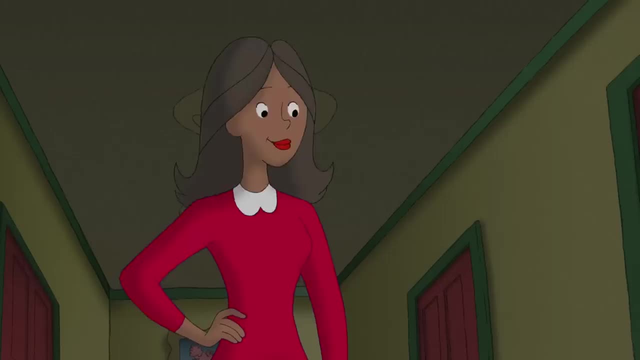 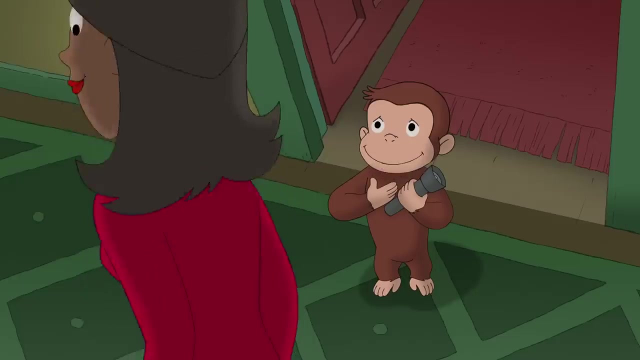 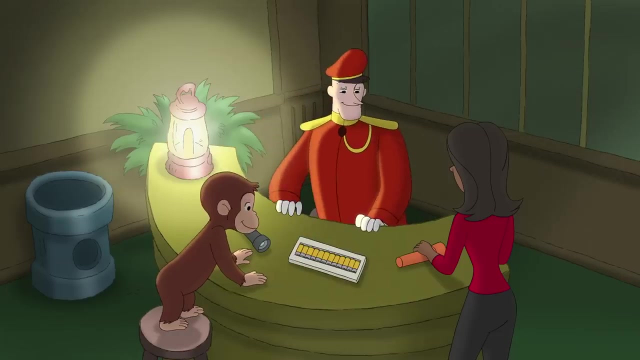 Oh, Uh-uh, Quack, quack, quack, Uh, Uh, Oh, Uh, Uh Uh. Then he must be in the lobby. I need batteries for my flashlight Batteries. Sure, Help yourself. Thanks again for the tip about the safe space. 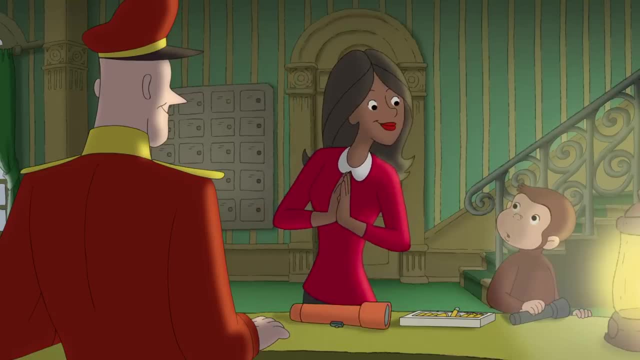 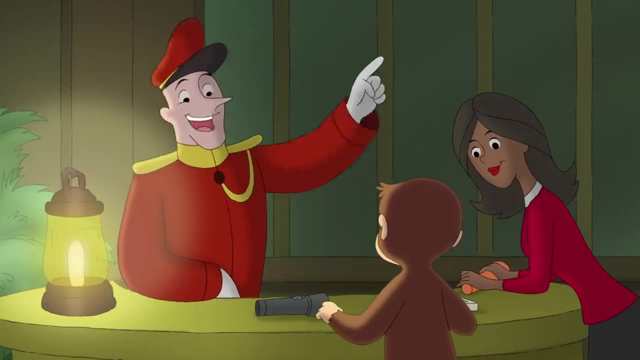 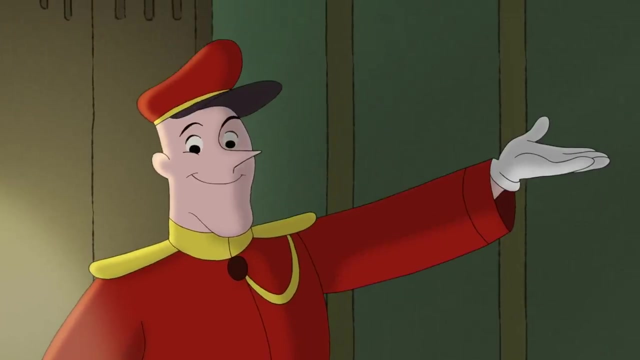 My dog has never been so calm during a storm. A safe space is a place dogs can go during a storm. They relax there because they can't hear or see the storm. That's why Hundley could sleep through the storm. The music distracted him from the thunder. 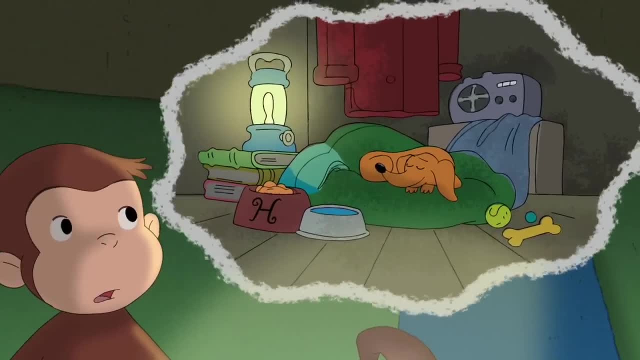 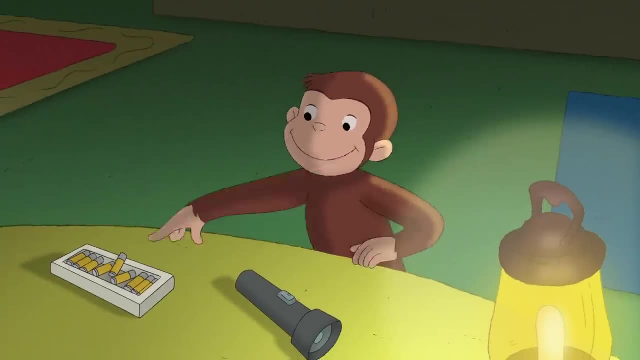 And he couldn't see the lightning from the closet. It was exactly what Charky needed. I'm going to sleep in the storm. I'm going to sleep in the storm. Take as many as you like, I've got tons of them. 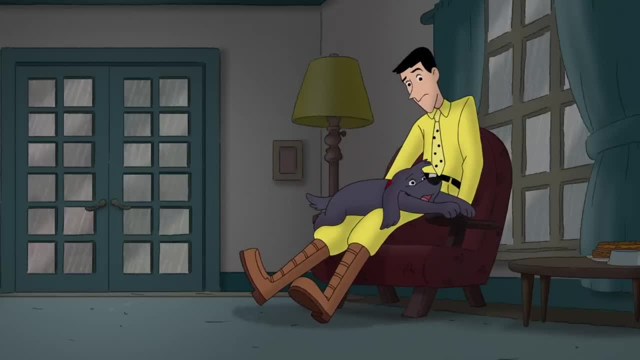 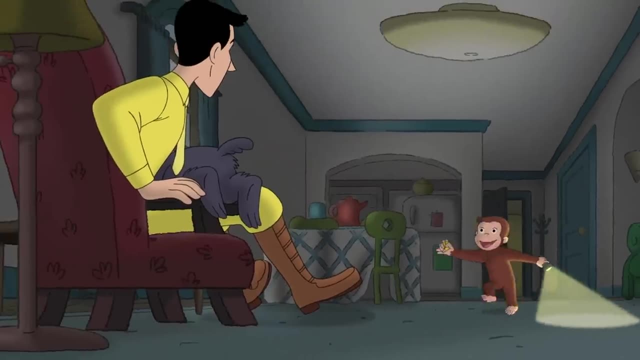 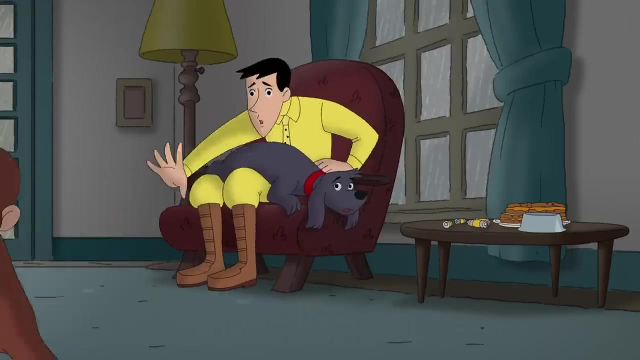 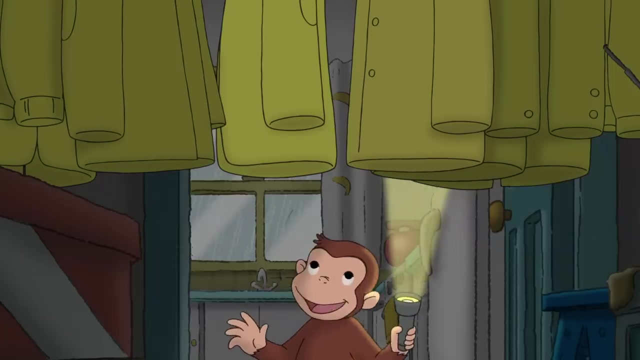 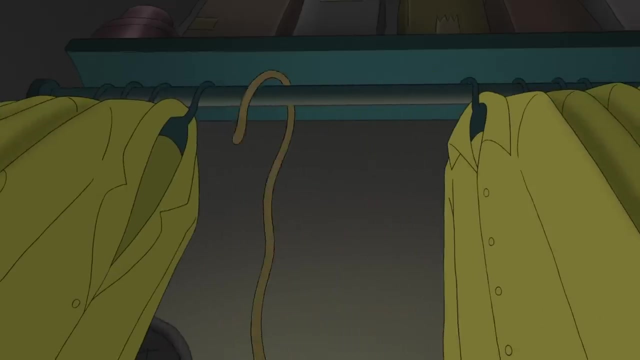 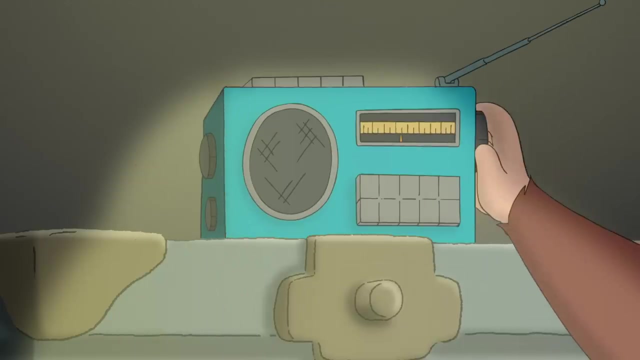 Hey Charky, how about I just stretch my legs? a little Boy, am I glad to see you, George? Wait I? A safe space needed a comfy bed. Um, George, Nice lighting, Soothing music. 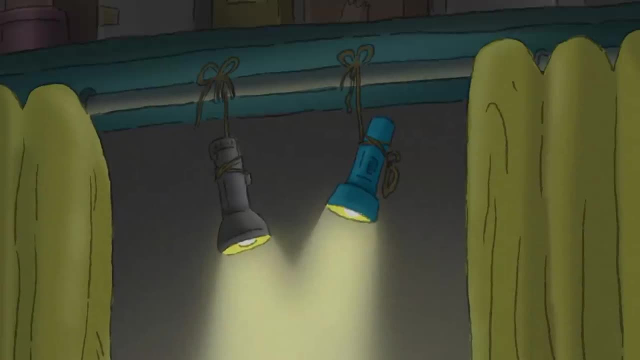 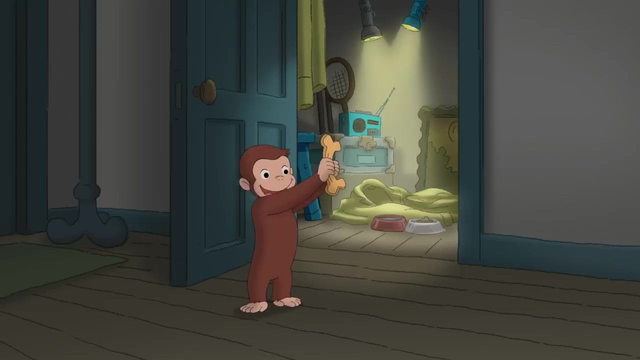 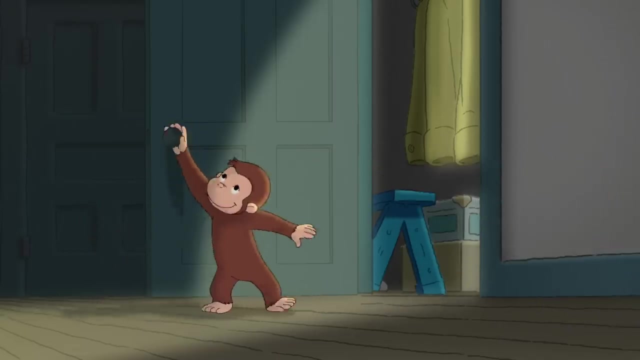 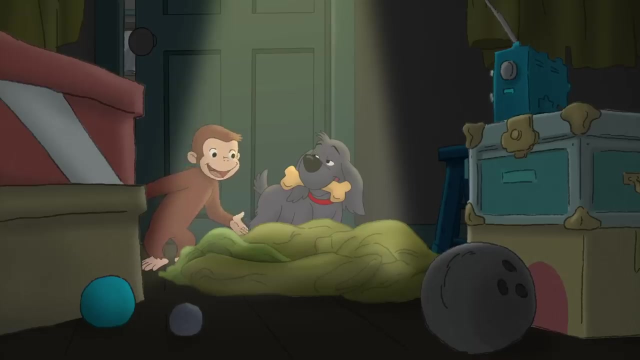 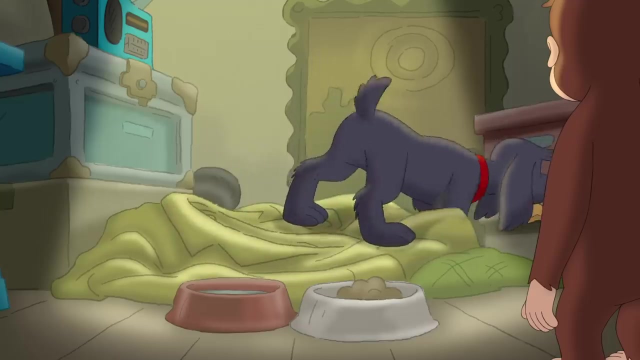 And snacks. One of the things Charky's safe space needed was: Charky, We can go to the party. Oooh, Oh, Oh, Oh, Wow. How about that? Oh Ooh. Finally, Charky was calm. 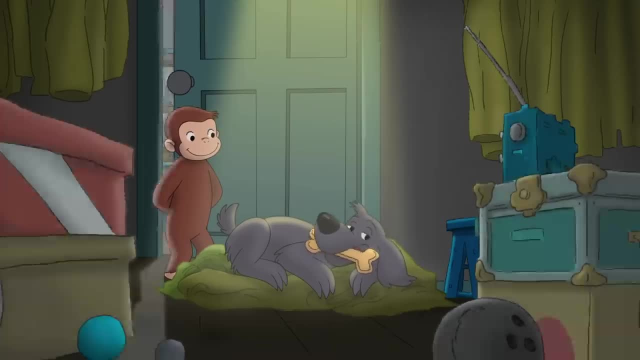 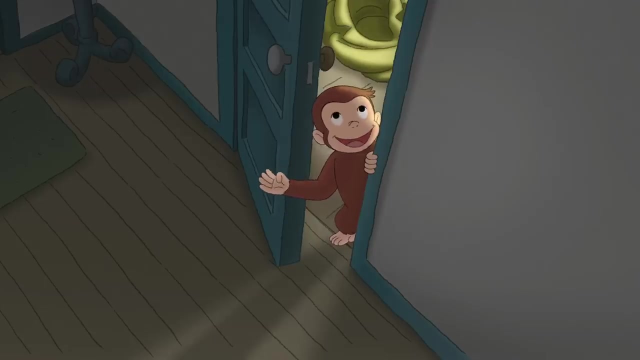 Ooh, ooh, Ooh, Ooh, Ooh, Ooh, おお. Oh, The time between the lightning and thunder was getting longer again. That meant the storm was moving away And Charky was happy The safe space had worked.